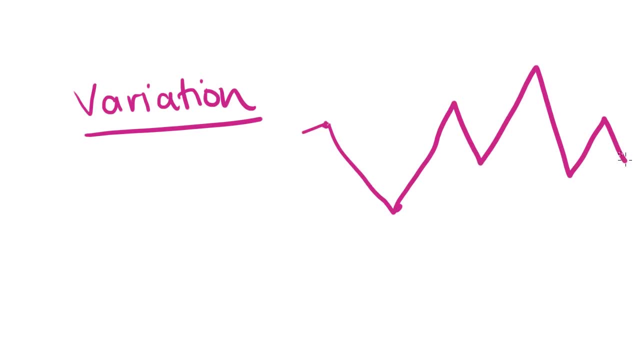 So high points and low points in the data. So here is a high point: each time It's like the top of the mountain, the peak of the mountain, And here's a low point: each time It's the bottom of the mountain, It's like a valley. So we're going to look at where the time series 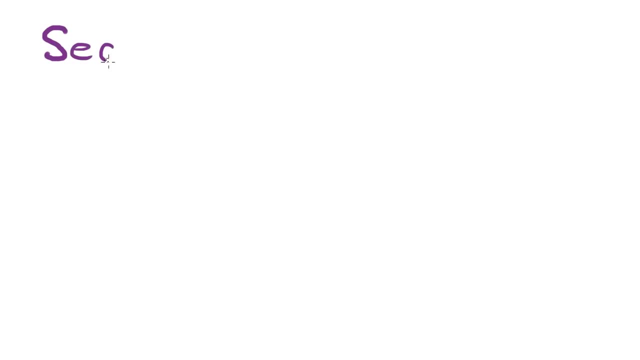 goes up and where it goes down again. The seasonal pattern, or seasonality as it's sometimes referred to, has regular peaks and troughs, And by regular I mean you could almost predict when they happen based on when they've happened in the past. You can see on this graph: we've got these peaks happening, but they happen at the same. 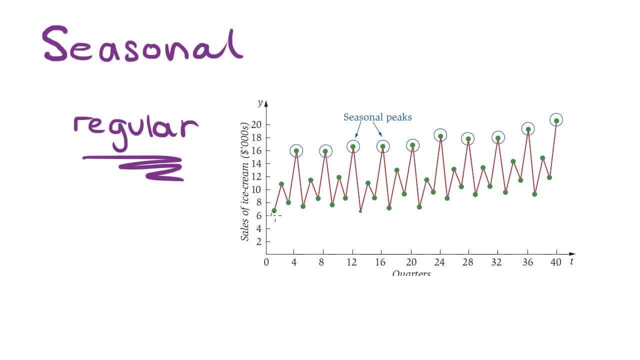 time each year. So this is quarters, and here we've got the first quarter. it's down, then it's up, then it's down, then it's a peak. And here we've got the first quarter: it's down, then it's up, then it's down, then it's a peak. 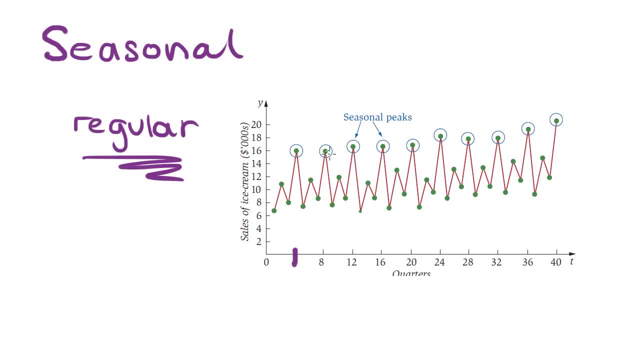 In the fourth, And then it's down, up, down, up. a peak in the eighth, And then it's down, up, down, up and a peak in the twelfth. So these peaks are happening every four quarters. 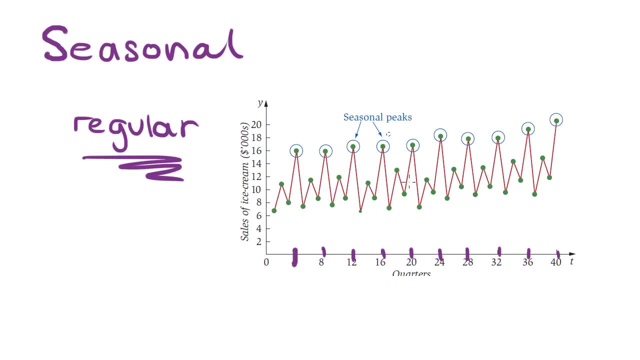 They're happening at a regular interval And so that we might attribute to the seasons- For example, four quarters of the year, that's seasons- autumn, summer, winter, spring. So perhaps this is ice cream sales or something like that. In fact it is- Look at that- sales. 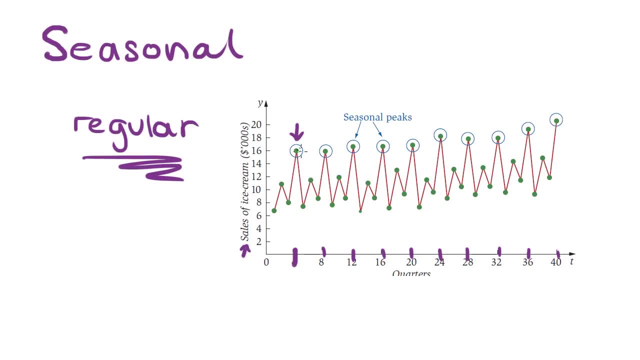 of ice creams. So ice cream sales go right up to the fourth quarter And then it's down, up, down, up a peak. So you can see that the sales go right up in the summer and they go all the way back down again in the winter. because who wants to buy ice cream in winter Now? 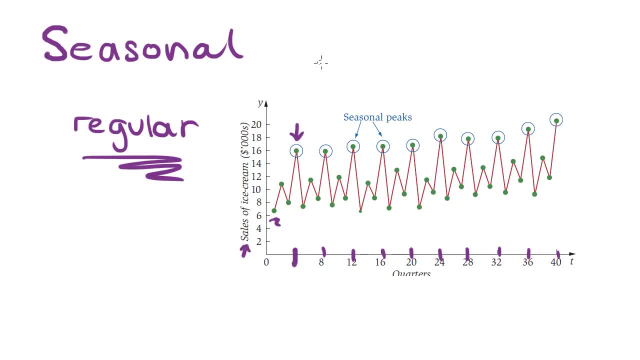 seasonality doesn't have to be tied to seasons exactly, So it doesn't have to be summer, autumn, winter, spring. It might be. if you have some weekly data. for example, your sales of something might always peak on a Monday and it might always trough on a Friday. And 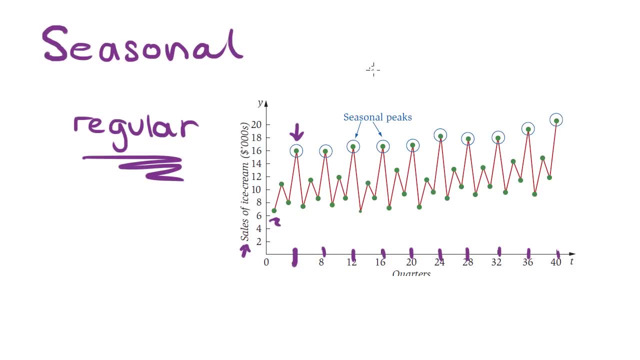 then if you put daily, if you create a daily time series, we'd be able to see: Monday is up and then Tuesday's down, Wednesday, Thursday, Friday, And then we've got Monday and then we've got Tuesday, Wednesday, Thursday, Friday, And then we've got Monday and then Tuesday. 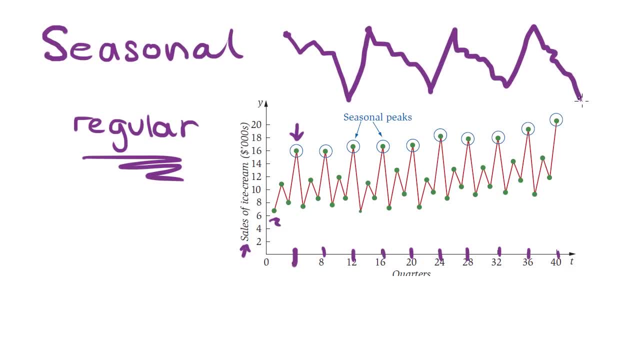 Wednesday, Thursday, Friday, and then we've got Monday, and then Tuesday, Wednesday, Thursday- Ooh, Friday is where it's down there- Monday and so on. So it's not necessarily seasons, it's just that it's regular peaks and troughs. This 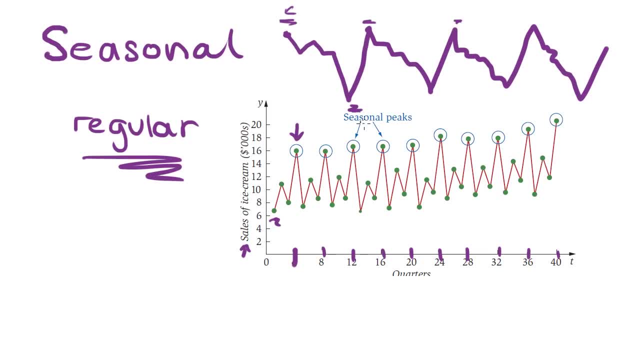 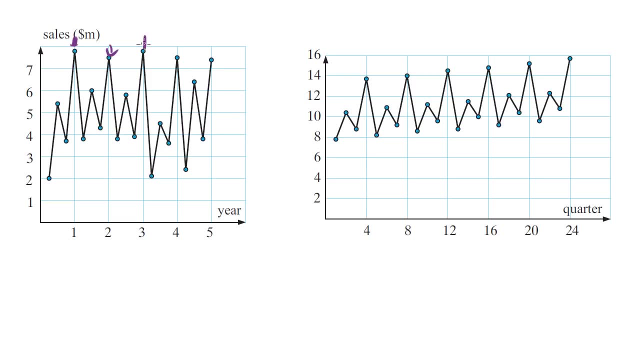 peak is always occurring on a Monday, this trough is always occurring on a Friday. Here's a couple of other seasonal examples. You can see here we've got some peaks happening, there's a peak, peak, peak peak, and we've got some troughs down here as well, where 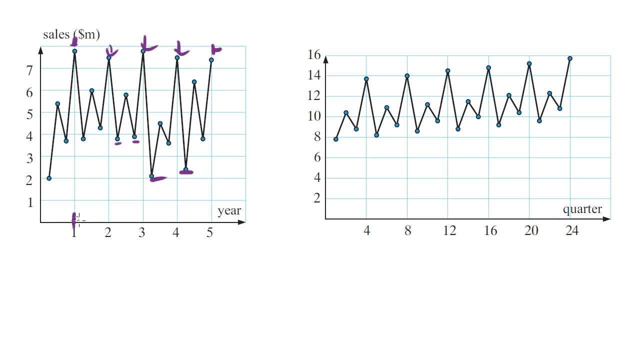 are these peak happening, peaks happening? this is happening right on the dash of the one year and this one's happening right on the dash of the two year. this one's happening right on the dash of the three, four and five. so if we had six here, we could pretty reasonably predict that that might be high up here as well. 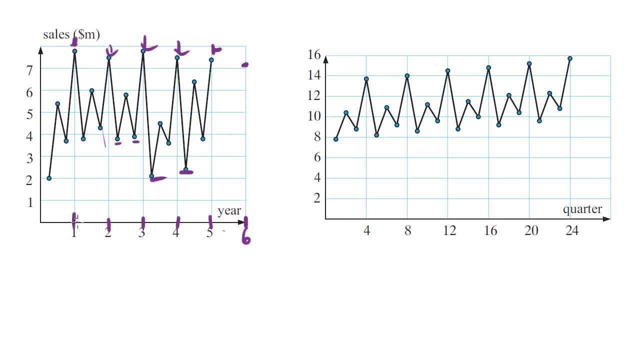 it'd be another peak, because that always happens at this dash, the in between sections. here we have a trough and then a high and then a trough, so it goes down, up, down in between and can you see how that's repeating down, up, down, down, up down for this interim part of the scale. so this is seasonal because we 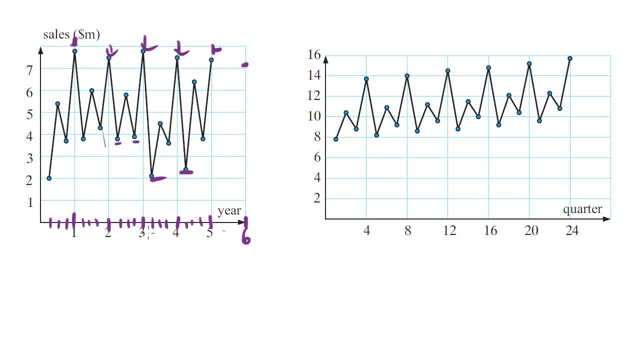 can see regular peaks and troughs, and they're occurring at sort of expected times in the time series. they repeat their pattern over and over, at the same time each year, or at the same time each month, or at the same time each week within the cycle. they repeat over and over with consistency, this one's seasonal over. 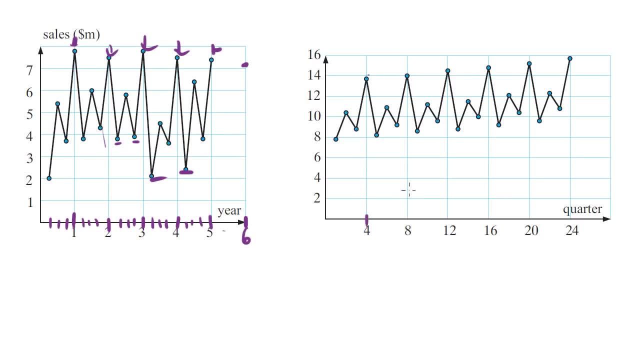 here as well. we can see: this peak is happening at the fourth quarter, this peak at the eighth, this peak at the 12th, this peak at the 16th, this peak at the 20th, this peak at the 24th. so every four quarters there's a peak, and these troughs 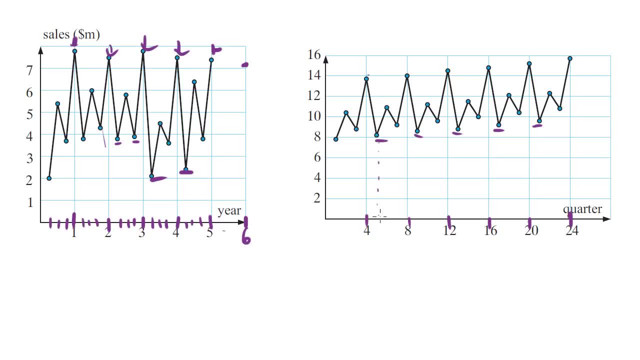 are pretty regular too, if you have a look at those: that's occurring at five, that's occurring at nine, that's occurring at 13, that's occurring at 17, that's occurring at 21. so there's a little dip, there's a trough, there's a valley at the same time in each of these. 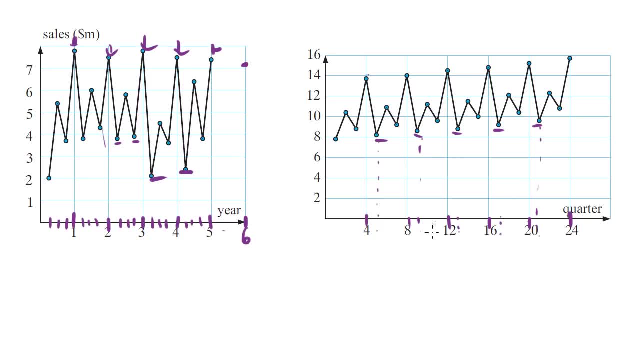 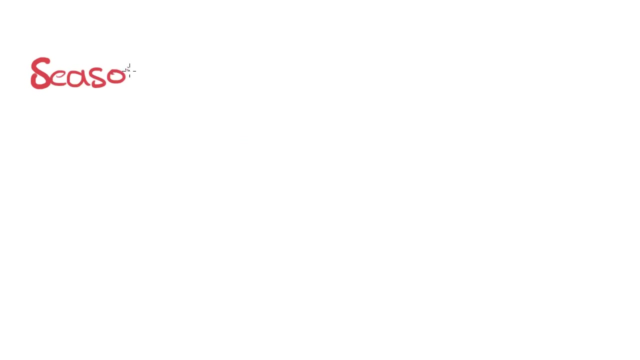 time series cycles as, if you like, each time. the other thing that this graph has is it actually has an upward sort of a trend. can you see that? so this is seasonal and it also has an upward or a positive secular trend with seasonality. so a seasonal time series has peaks and troughs that are at. 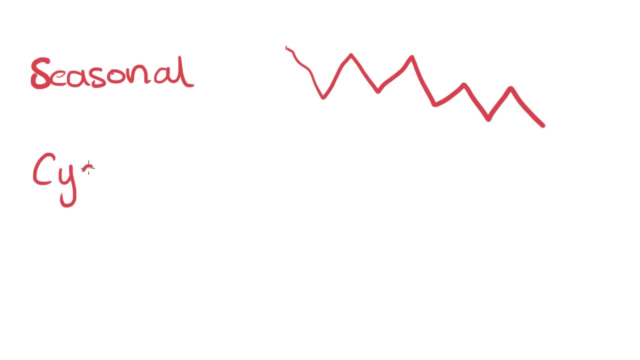 predictable times. cyclical or a cyclic time series plot has peaks and troughs, but they're at unpredictable times. so this one will still have a shape where you can see mountains and valleys, significant ups and downs, but you can't predict when they're going to happen. they don't happen at regular time. 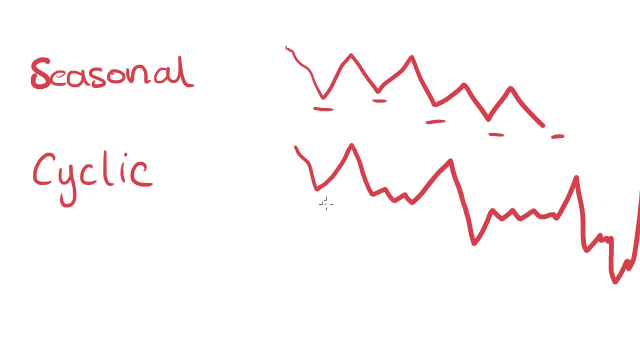 intervals. they just happen whenever. so, for example, a share price might go up like this when you hire a new CEO, and then it might go down like this when you sell off a part of the business and then it might go up like this because you know you acquire some new business, something like that. this peak didn't. 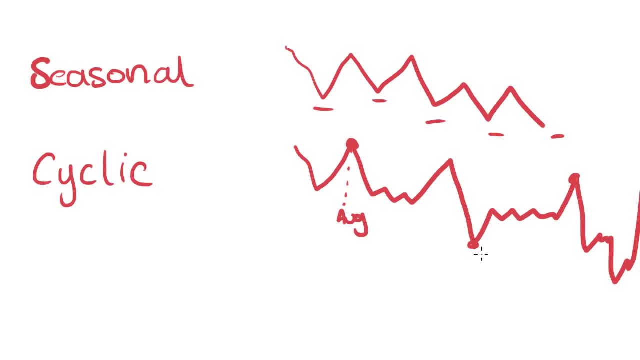 happen because it's August, you know. this trough didn't happen because it's January. this peak didn't happen because it's, you know, February. the peaks and troughs happen for other reasons, and for because of that, you can't predict, according to time, when they're going to happen. there's still a trend that goes. 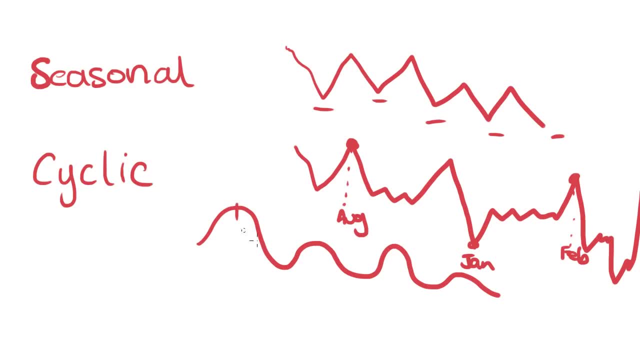 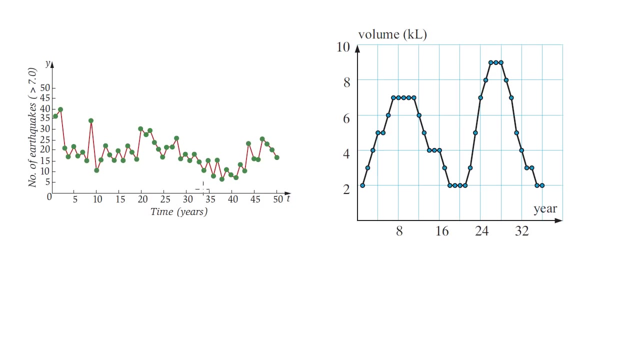 like that up and down generally, but the time gap between them isn't the same each time. so the difference between seasonal and cyclical is the predictability of the peaks and troughs. cyclic time series plots might look a bit like this: here's some peaks and troughs: peak, trough, trough. 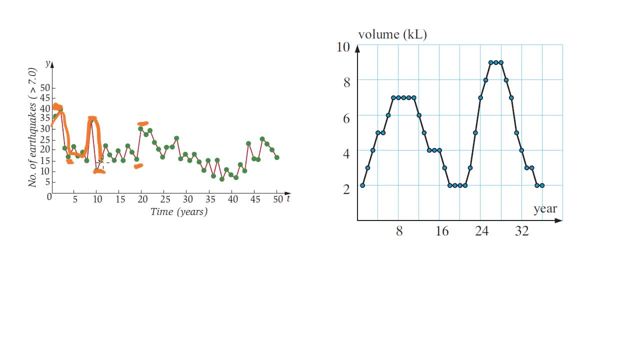 peak. so this one's here is going up and then down and then up, down and then up and then down and then down, down, down, up and then down and up. so we've got peaks and troughs, we've got a mountain range going on here, but they don't occur at. 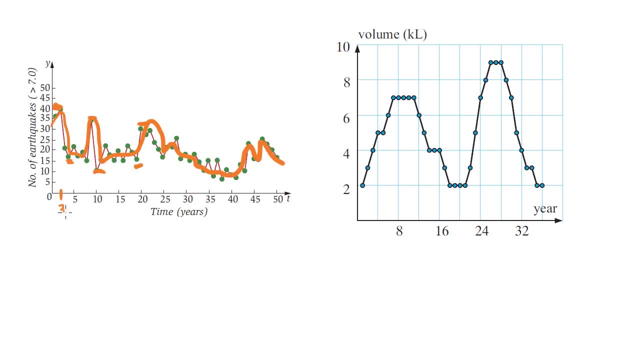 regular intervals. this one's occurring it. what's that? three maybe, and then the trough is at four, and then this peak is at ten, and then this trough, this trough. this downward part of the trend is longer than this one, and then this downward part of the trend is much longer so. 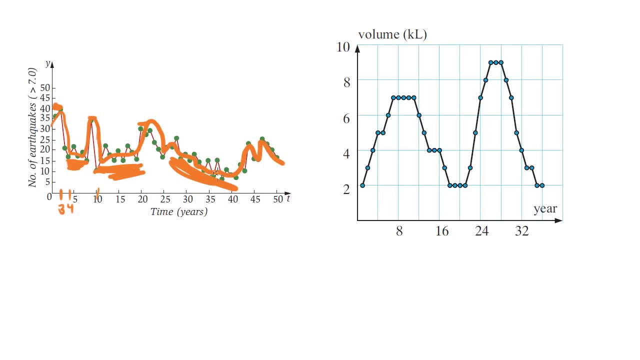 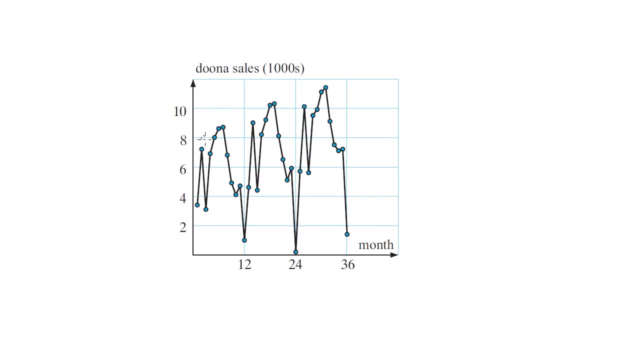 there isn't a regular gap between all of these peaks and troughs. over. here again, we've got a clear sort of shape, we've got our mountain range, but the time that they're occurring isn't regular. having a look at this example, do you think it's seasonal or cyclical? cyclical? let's have a look at where these peaks 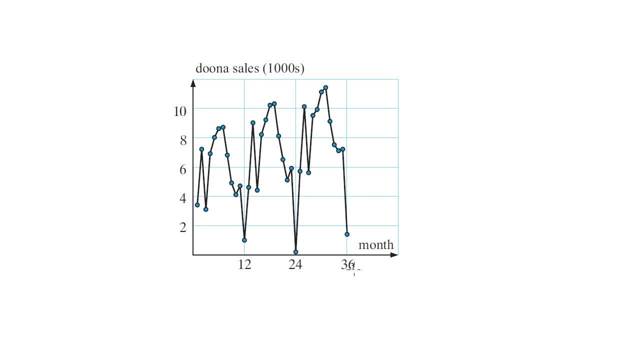 and troughs are occurring. we've got months going along here: 12, 24, 36, so that's at the end of the year, that's at the end of the year and that's at the end of the year. and what do you know? the same time each year, there's a bit of a 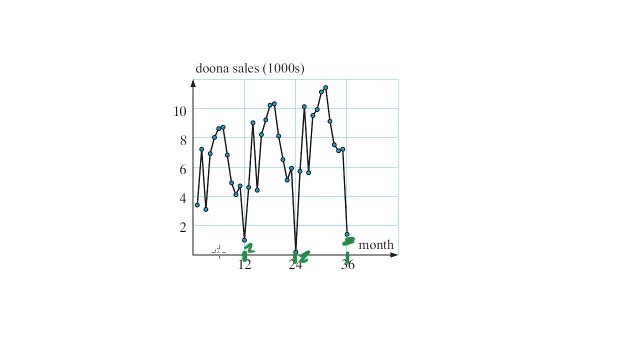 trough. what about where these peaks are occurring? that peak looks like it's happening about halfway through the year. what happens about halfway through this year? oh, what do you know? there's another peak. what happens about halfway through this year? ah, there's that peak again. so this is seasonal. 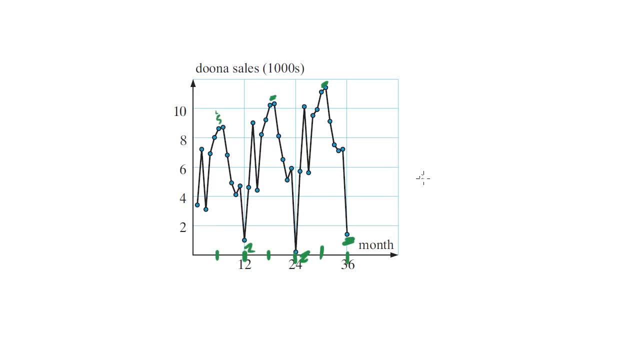 because these peaks and troughs are happening at the same time each year. the other thing that this graph has is a sort of upward kind of trend. even though these troughs down here are pulling it down this way, overall, over time it's going up the page. so this one has a positive trend and it's seasonal. another: 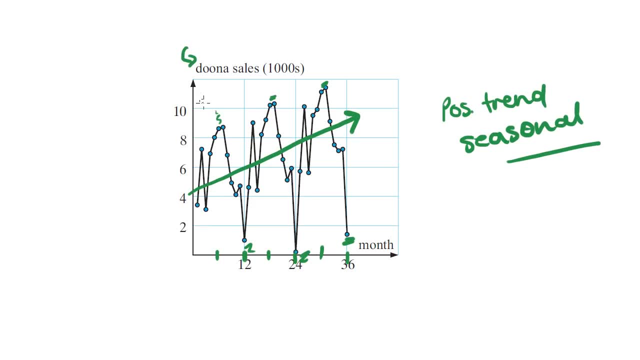 way. that would have been useful to work that out. if you have a look at what we're actually measuring- doona sales- it makes sense, before you even look at the graph, think about the sales of doonas. what would they be like? they probably have a high point right in the middle of the year. 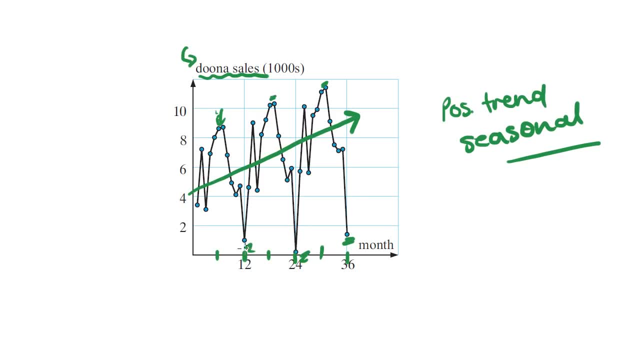 when it's winter, and they probably don't sell very many of them at the end of the year, when it's summer, when it's hot, which makes sense. here too, these little troughs so with, before you even look at the time series plot, sometimes you can. 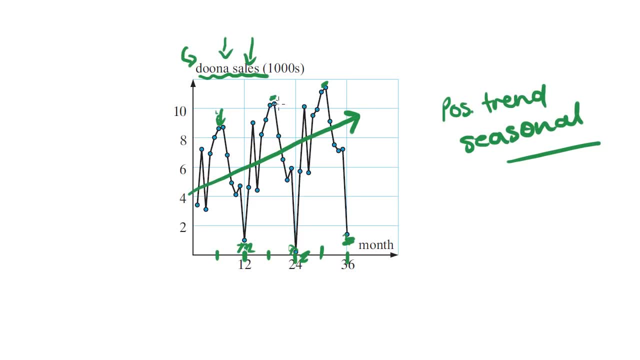 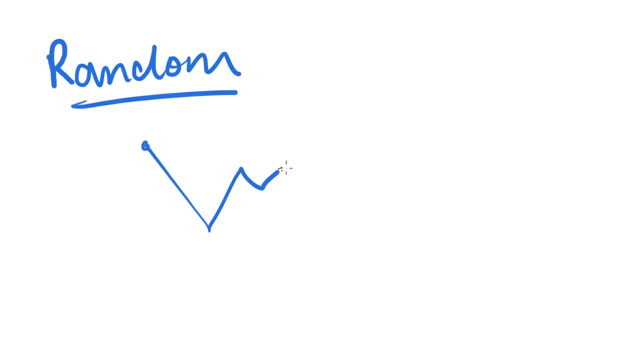 predict whether something might be seasonal, cyclical or random. a random time series plot doesn't have any obvious peaks and troughs happening for particular reasons. it's basically what random sounds like. it's just all over the shop. seasonal: you can predict peaks and troughs. cyclical: it has peaks and 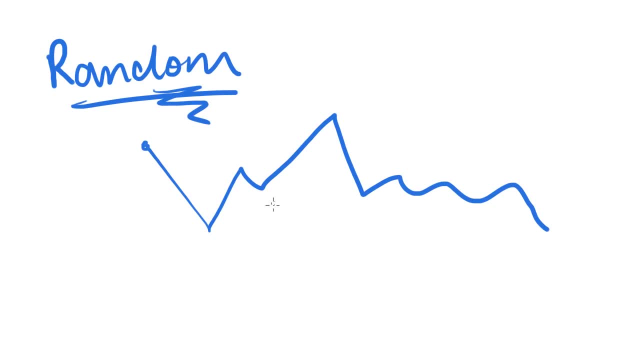 troughs and they're just. they occur for different reasons other than time and random doesn't really have an obvious sort of pattern of the variation to it. the variation is just all over the shop. there could be a trend upward or downward, with the variation being random, but in general you. 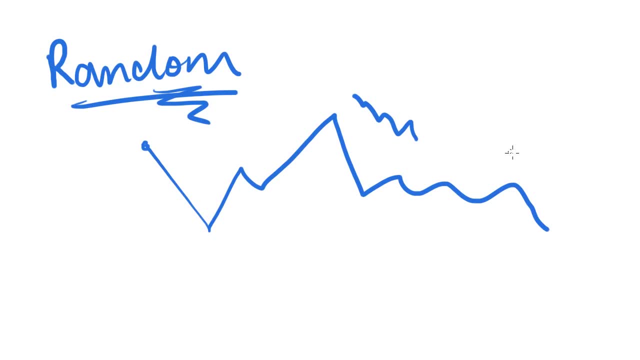 don't see a pattern of peak and then trough and then peak and then trough. here are two examples of random time series plots. this one here doesn't really have any significant piece peaks or troughs until about here and that doesn't repeat at any other point in this time series. so it's random because it's kind of all. 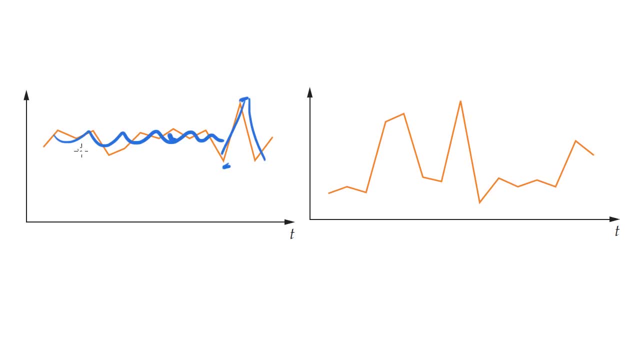 wavy along there and then there's this going on. there isn't an obvious up-down, up-down, up-down to it. this one here has a peak and then a peak, but then it doesn't repeat again over here. it sort of breaks its own pattern. so this: 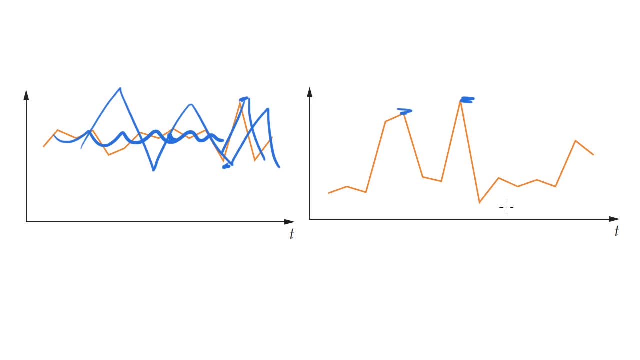 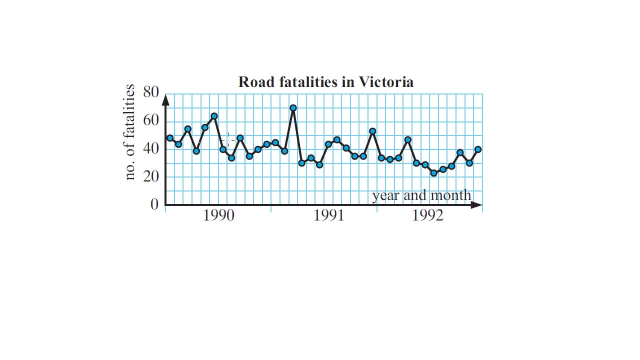 variation is random, because there isn't something that's really repeating itself in any significant way. what can we say about this time series? is there any sort of pattern to it? can we see an obvious pattern of peaks and troughs? well, here there's a peak and here there's a peak, but it doesn't really look like there's. 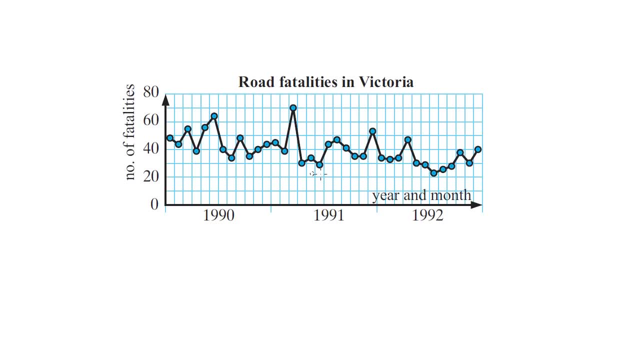 any sort of pattern to it. there's no rhyme or reason for why things are going up and then down and road fatalities. in Victoria. you wouldn't expect to have regular peaks and troughs either, but this one does have a sort of downward trend. as time goes by, this is all generally decreasing, so there's no. 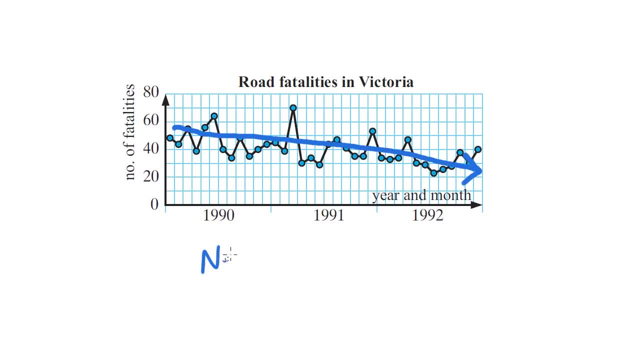 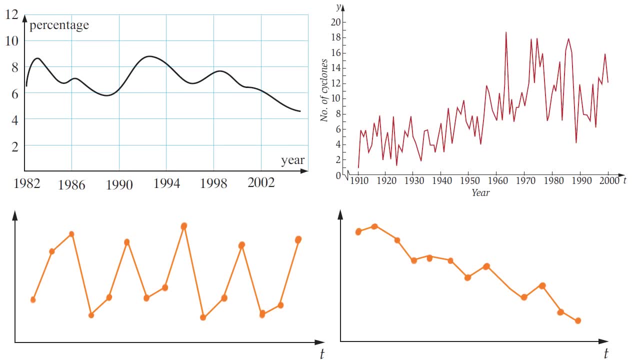 pattern to the variation, but there is a negative secular trend with random variation. let's look at a fourth time series plots. have a look and see if you can work out what the pattern or trend to these might be. so this first one: here you can see that it's got a peak and a trough: peak trough, peak trough. so it seems like it. 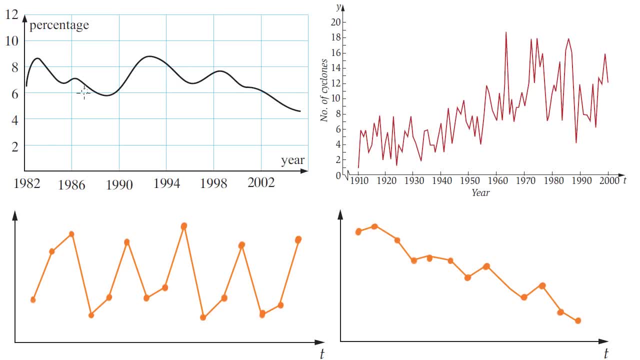 does have a pattern to that variation. it's doing the same thing over and over, but it's not doing it at regular intervals, so that would make this one cyclic. what about this one down here? it's going down, up, up, down, up, up, down, down, up, down, down, up, down, down, up it. 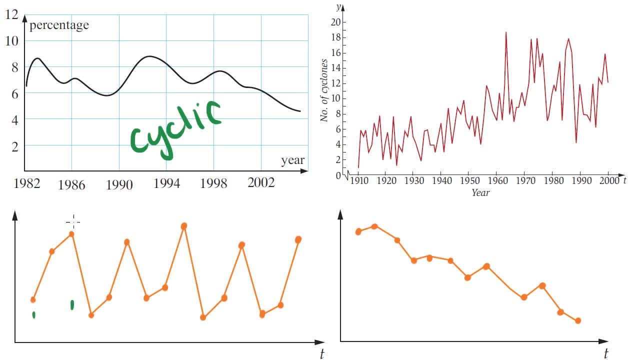 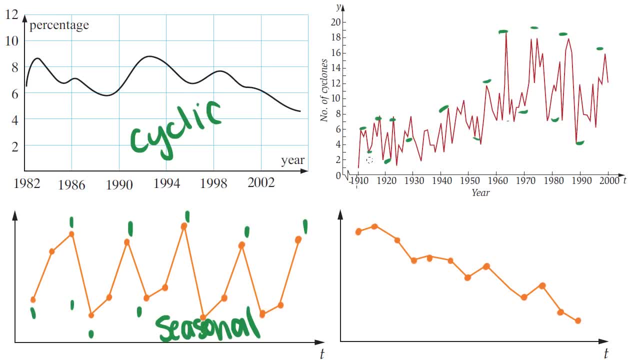 down up. it's doing something over and over. it's got a pattern to it, but there isn't an even space between each one. there isn't predictability to when these ups and downs are going to occur. so this one is cyclic. what about this one? it's 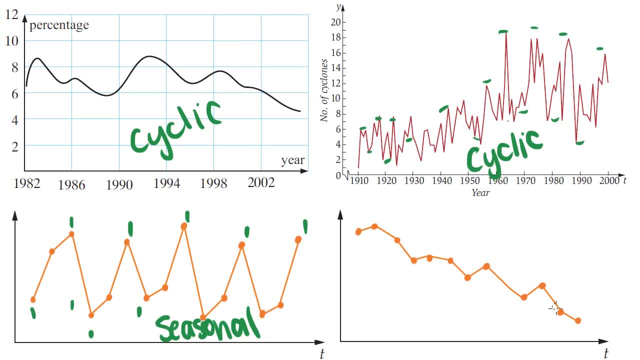 going down up, nothing really significant. with the down up stuff here, the peaks metrics aren't really standing out to me, which means there isn't much variation going on with that. the variation there is probably just random, but there is a definite trend going down the page. so to describe this one, i would say it has a negative secular trend. this one up. 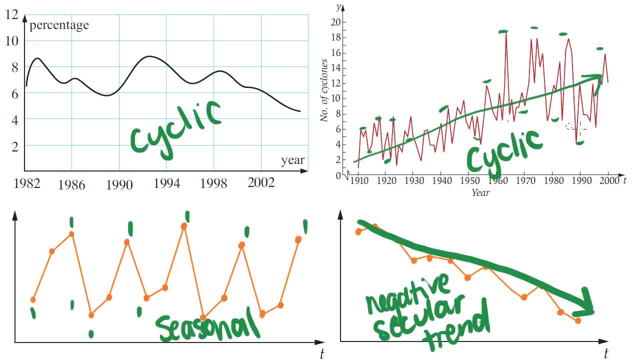 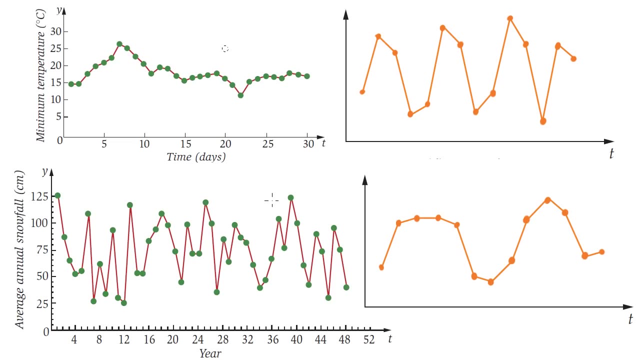 here also actually has a trend generally going up the page, so that would be something worth talking about. this one here has an ever so slightly negative trend, And this one here doesn't have a trend. It's not really going up or down, It's basically staying the same. And have a look at these four time series plots and see if you. 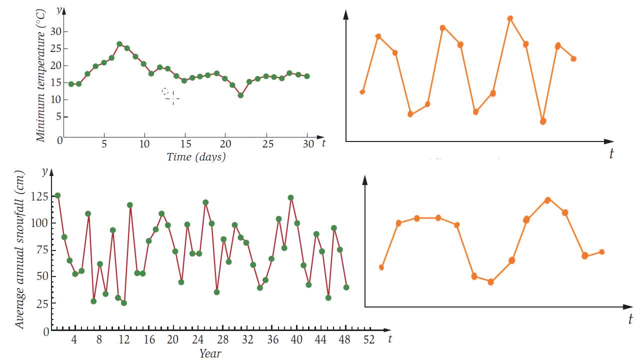 can work out what's going on with them. Let's start with this top left one. Is there any significant pattern happening with peaks and troughs? There is one peak here and then a bit of a trough here, but there isn't something that's repeating, because we can only see one peak and one. 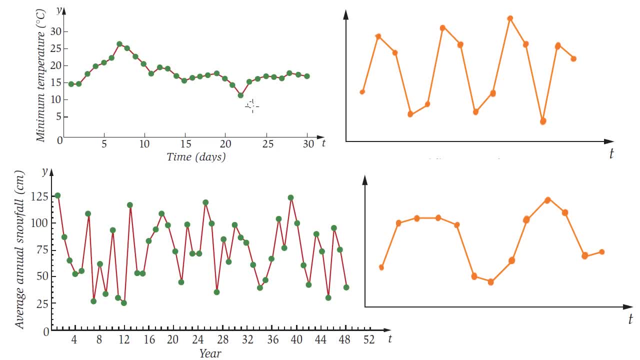 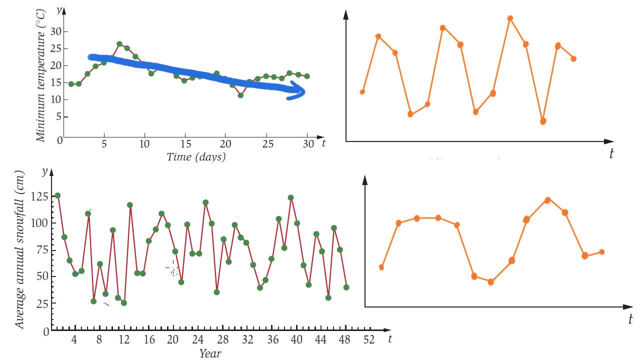 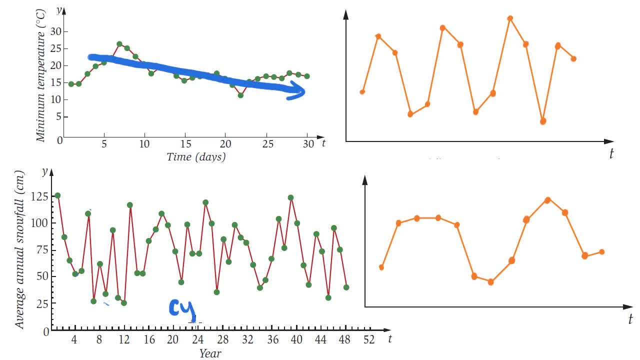 It just goes up and down at different times, which means that this one is cyclic, cyclic. And what's the trend? Is it going up the page or down the page? It's kind of hard to tell. If anything, probably slightly upward. What about this one on the top right? I can see peaks and 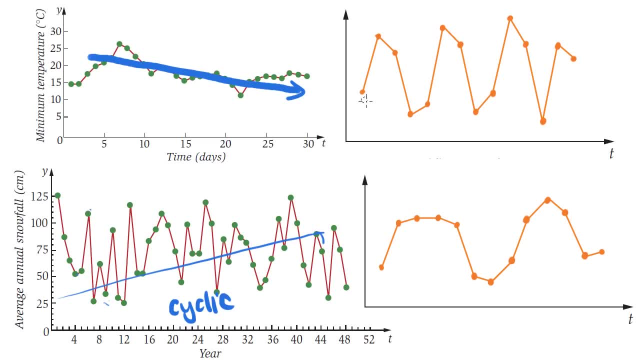 troughs, peaks and troughs, peaks and troughs. And what do you know? It's going down, up, down down, And what do you know? It's going up, up, down down, And what do you know It's going? 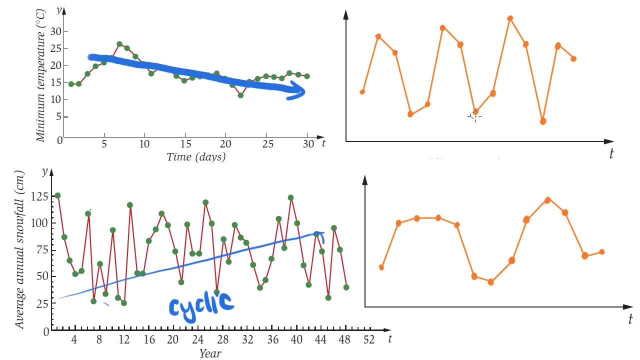 up, up, down, down, Up, a little bit up, a lot down, a little bit down a lot. Up a little bit up, a lot down, a little bit, down a lot. And if you have a look at the distance between these peaks, that's occurring at regular intervals. And the distance between these troughs is occurring at regular intervals as well. So this one is seasonal And, if anything, there's a slightly upward trend to it, But that's not too obvious. And what about this last one? Any obvious peaks and troughs? 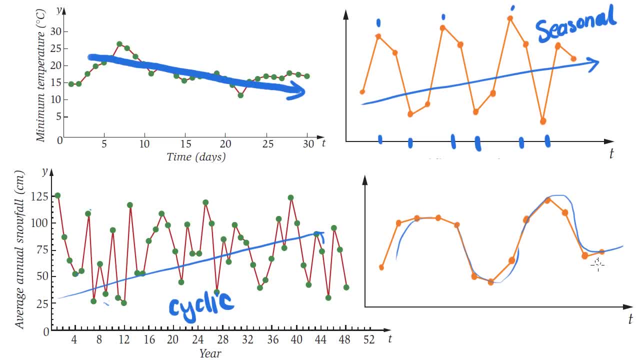 Yeah, obvious peak, obvious trough. obvious peak, obvious trough. So there's a pattern to it. Now, how regularly is that occurring? Is that occurring because of time or because of something else? So this peak here, and then it stays high for another three sort of time periods And then we go low for three time periods. So there's four periods in that peak and there's only three in this peak And then there's two down here. It doesn't look like that's a repeating pattern. 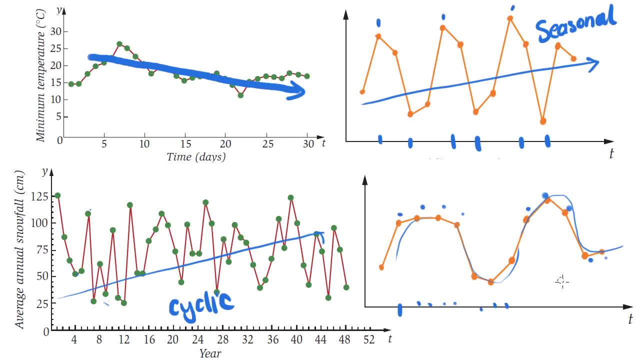 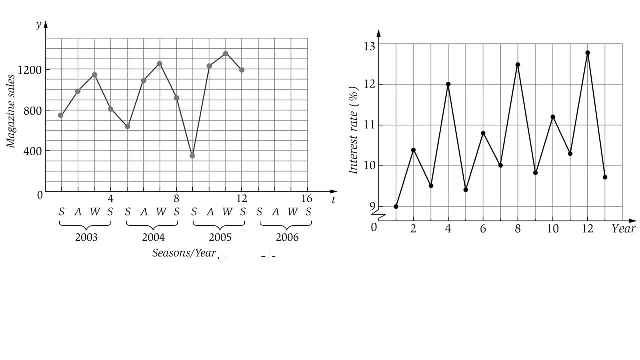 Due to time, It looks like those peaks and troughs are occurring because of something else. So this one's cyclical, It goes in cycles. A couple more examples. Let's see what's going on with these. This one here has got some obvious peaks and troughs happening, And where's this peak happening? That's happening in winter. We've got summer, autumn, winter, spring here. Then we've got a trough happening in summer, And then we have another peak happening in winter again. Okay, and then another trough happening in winter. 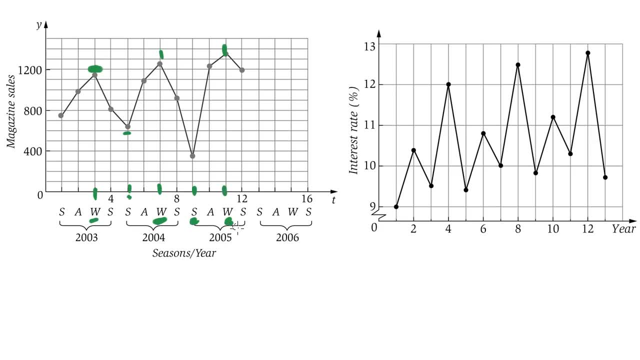 And a peak, let me guess. Oh, what do you know? It's happening in winter. So probably what would happen over here? we would be able to fill this in a little bit and say, well, there's probably going to be a trough in summer somewhere down here, like this, And then there'll be another peak in that winter. It'll get higher again, maybe up there. So this one is seasonal. And what about this one on the right? Is there any regularity? I can see the peaks and troughs are occurring over and over. And when are these peaks and troughs occurring? 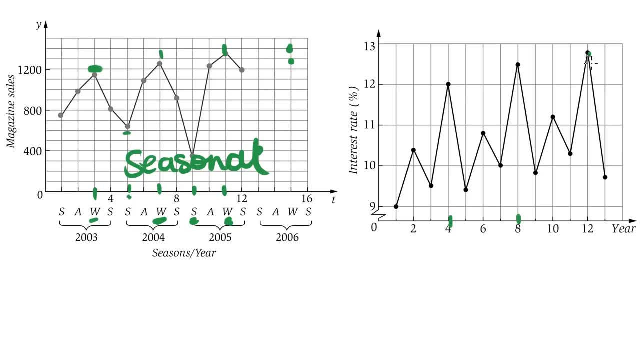 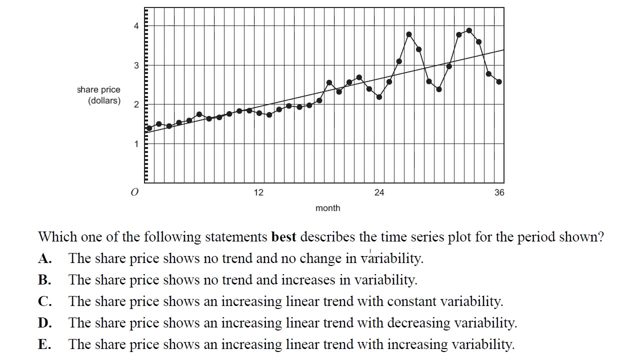 That's at four, then that's at eight, then that's at 12.. Okay, it sounds like it's happening every four years, And these troughs are occurring immediately after that peak as well. So this one is seasonal as well. And the other one that this thing has is that trend. Can you see how it's going up the page as we progress? It's got that positive secular trend. And lastly, here's how this gets tested on the exams. This is from the 2005 exam. one 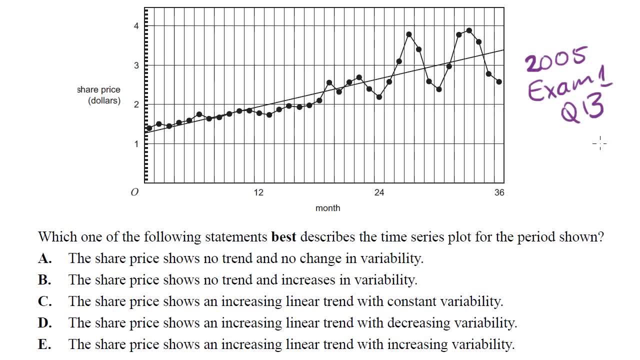 Multiple choice And it was question 13.. The question said which one of the following statements best describes the time series plot for the period shown? So, looking at this time series plot, okay, the share price shows no trend and no change in variability. Well, it's not going to be that, because I can already see there's this trend line on there. It's got a positive trend to it. See that positive going up the page along here, that trend. So it's not going to be this one that says no trend. 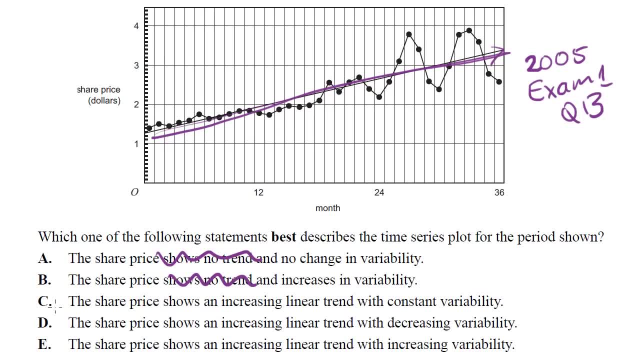 And it's not going to be this one which says no trend. So it's going to be one of these three that says the share price shows an increasing trend. The other options are constant variability, decreasing variability or increasing variability. So let's have a look at the variability. The variability is these peaks and troughs. So along here it's conforming to the line. It's not moving around very much. It doesn't have really fluctuating peaks and troughs, And then it starts to get a bit more variable. It's got a peak trough, peak trough. 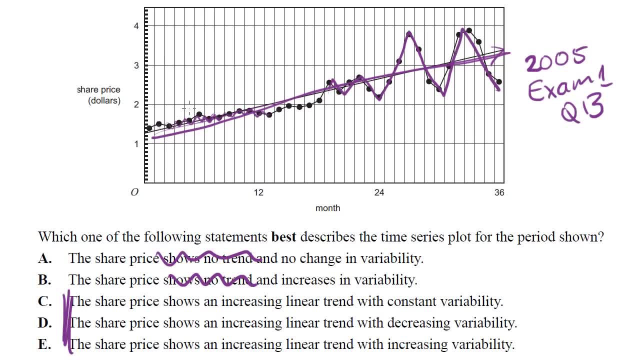 And then it's got a huge peak, huge trough, huge peak, huge trough. So while it was little variability here, it started to get bigger and bigger as we went along. So it shows an increasing linear trend and the variability is increasing over time. So the answer here is E. 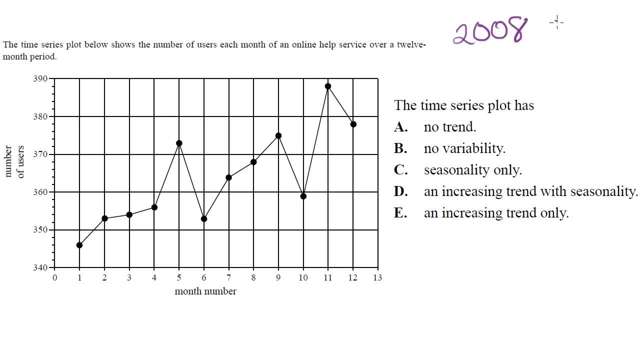 And finally, this question appeared on the 2008 exam, one multiple choice, And it was question 11.. And the question said this: The time series plot below shows the number of users each month for an online help service over a 12 month period. So what do you notice about this time series? To me, it looks like it's going up the page, like that. It's got a bit of a positive trend to it. That's the first thing I notice. Then I noticed some significant peaks and troughs happening here, So I'll investigate that. Now, what does the question say? The time series plot has: A- no trend. Well, it's not going to be that, because there's clearly a trend going across the page, So let's rule that one out. B- no variation. 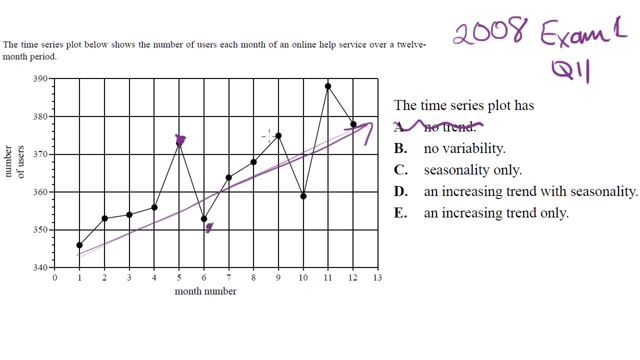 C: variability. I can see peaks and troughs and peaks and troughs and peaks and troughs, So there's variability going on there. So it's not that one. Now, our other options are seasonality only, an increasing trend with seasonality, or an increasing trend only. So let's have a look and see if there's seasonality there. First of all, we can probably rule out C, because C is about there being only seasonality. So let's rule that out because we've got this increasing trend.